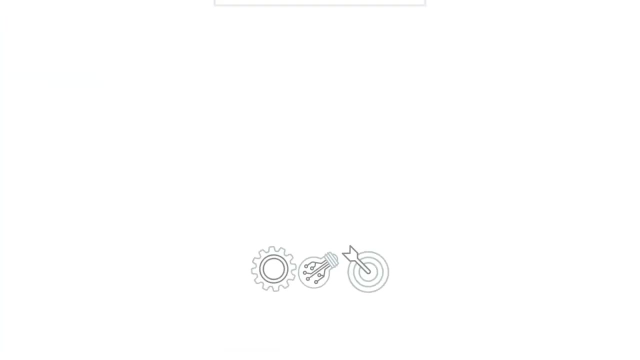 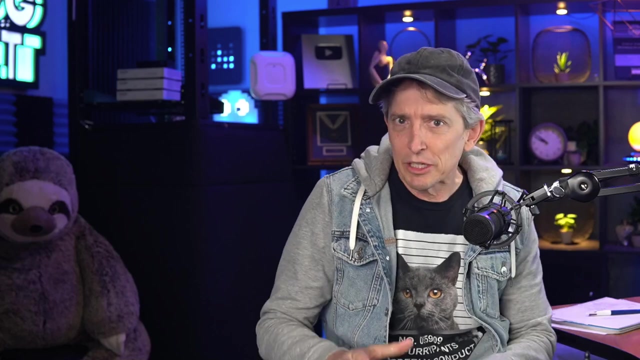 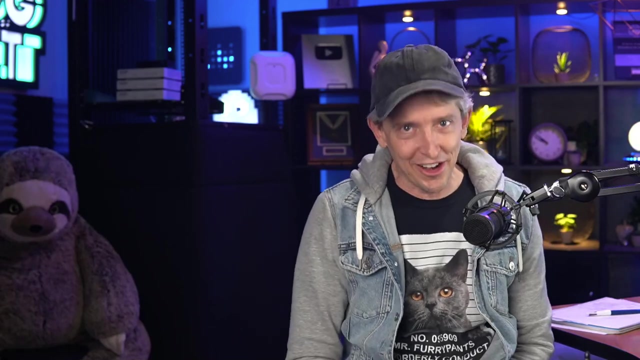 Hello and welcome. My name is Keith Barker And in this video we're going to take a look at some network topology designs, not the five tier or the four tier or the one tier, but rather the two tier and three tier hierarchical models. So let's begin with. 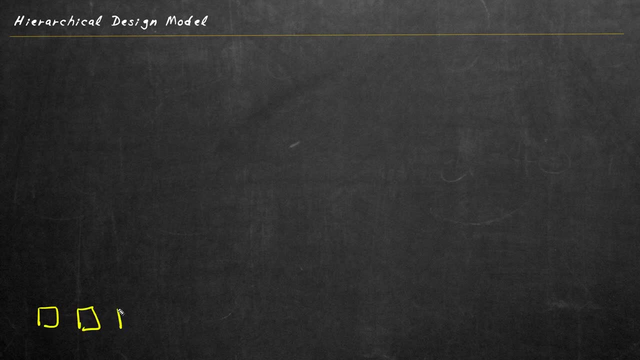 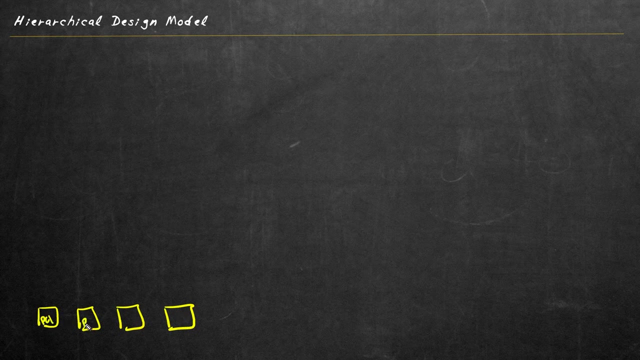 something that everybody knows, and that is a device like a computer that needs access to either the internet or internal servers. So this will represent four computers: We'll have PC1, PC2, PC3, and PC4. And those can be Linux devices, Windows devices, Mac devices, 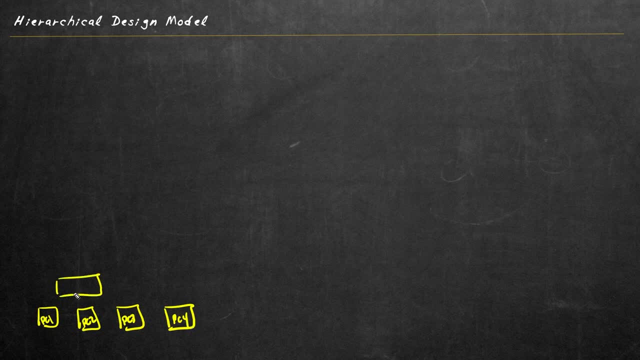 just computers that are on a network And as far as the connectivity goes, those devices are very likely connected to some type of a layer two switch. So let's call this switch one and switch two, And then they've got some connectivity to those switches. So for these computers that are 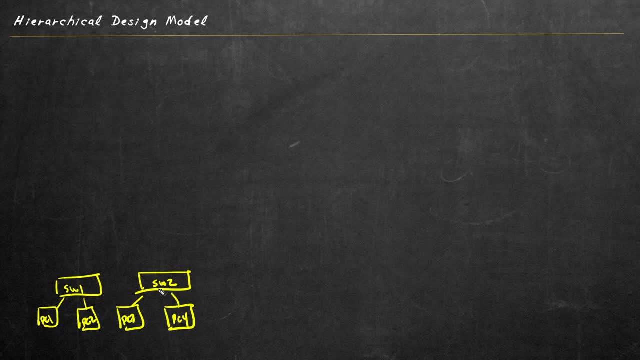 getting access to the network. you could say that these switches are their on-ramp to the network. That's how they connect. So I'm going to go ahead and draw a little rectangle around these and I'm going to give this a label. I'm going to call it the access layer Again. 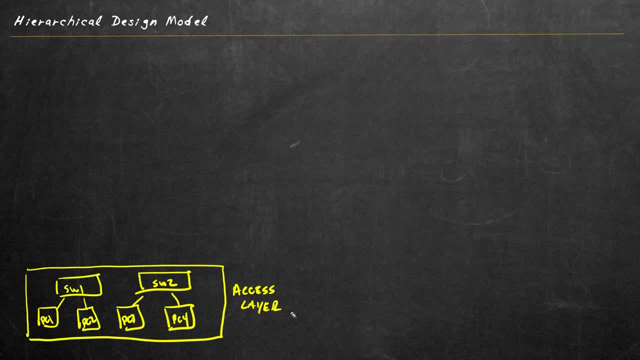 think of the access layer as where the devices are accessing the network, where they get onto the network. So let's imagine this access layer supports four different VLANs. And so let's imagine PC10 is in VLAN 10,, PC2 is in VLAN 20,, PC3 is in VLAN 30, and PC4 is in VLAN 40. And the way 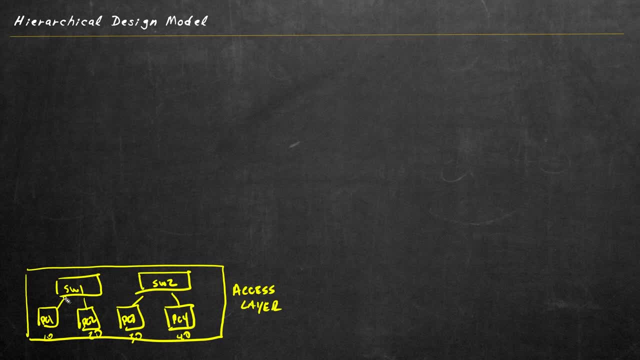 we control what VLAN these PCs are in is by configuring these switch ports. So on switch one on this port, we'll call this port A. We assigned it as an access port. on port B, we assigned it as an access port for VLAN 20, and PC3. on port C, as an access port for. 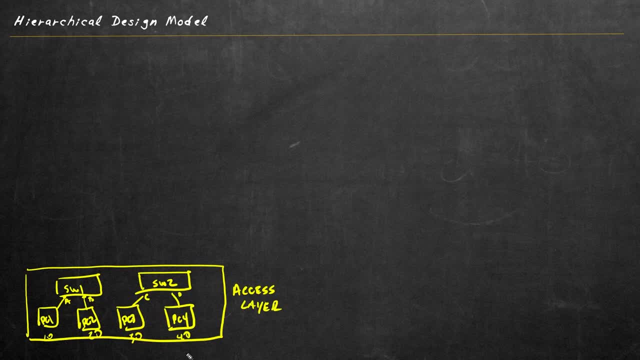 VLAN 30, and on port D, as an access port for VLAN 40. And for the IP subnets used for each of those, let's go ahead and use 10.vxx with a slash 24.. So the second octet here in our IP address will. 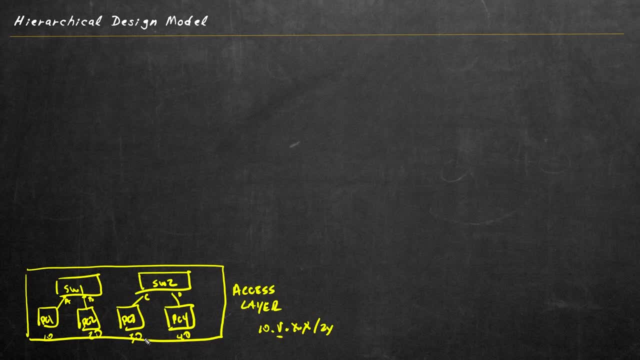 make it match our VLAN number. Although it doesn't have to, it is convenient from a design perspective to look at an IP address and know automatically what VLAN that's associated with. So PC1 would be on the 10.20 network, PC2 would be on the 10.20 network, and so forth. So while switch one 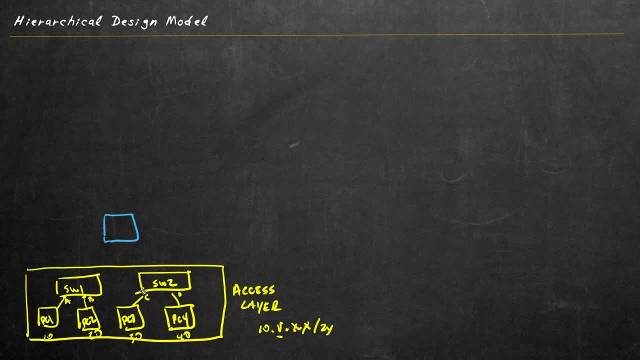 switch two are layer two switches to perform the routing between subnets. we need something that can do routing, which would be like a router or a multi-layer switch, and that's what we're going to put right here And we're probably going to want some fault tolerance. so I'll go ahead and 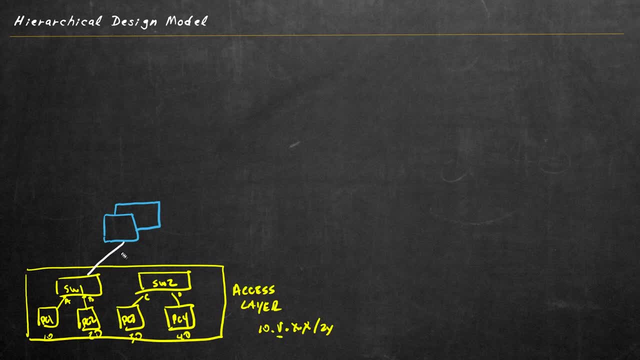 put a couple of them here And we'll put some connectivity down to switch one and we'll put some fault tolerance there. So I'm just going to draw this as redundant connections between switch one and both of these devices here And we'll do the same thing for switch two. We'll have some 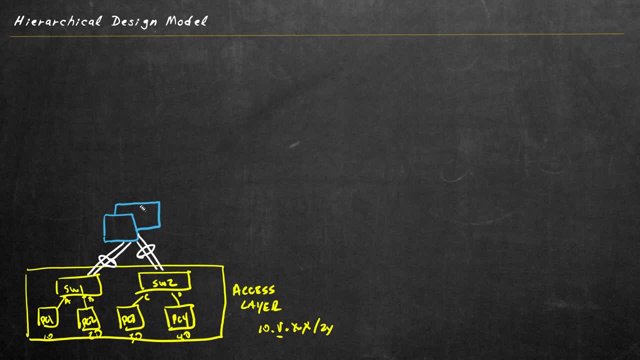 single link, It won't be a problem. So these devices here, these multi-layer switches, they're going to be responsible like kind of an aggregation point for all the VLANs that are here, if there's routing that's needed between VLANs 10.20,, 30, and 40. And they have a special name. 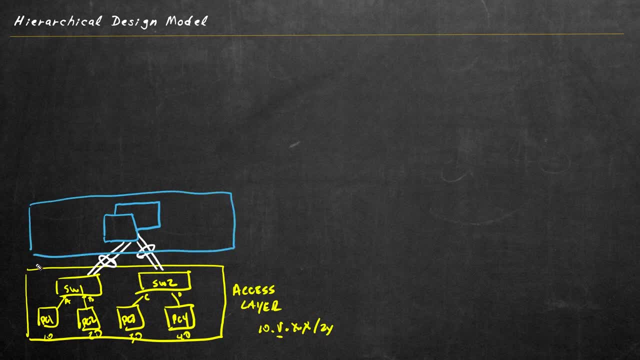 for these devices which are acting as the aggregation point, doing all the routing for these VLANs, and that's referred to as the distribution layer, And so I'm going to name these D1 and D2 for multi-layer switches at the distribution layer, So these could be two separate. 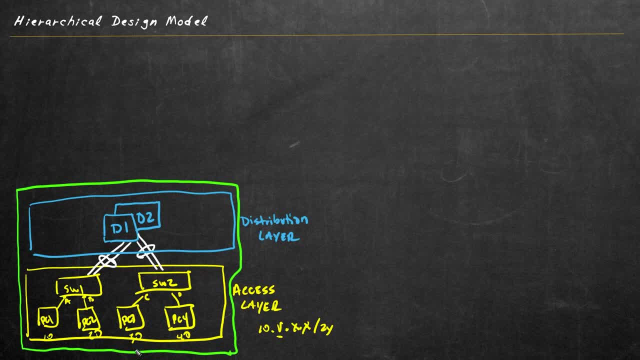 with ether channel between the two devices. Either way is great. So let's imagine: everything here in green represents maybe one building on a campus, and they have more than just one building. So let's go ahead and repeat the process over here. We've got some access layer switches. I'll 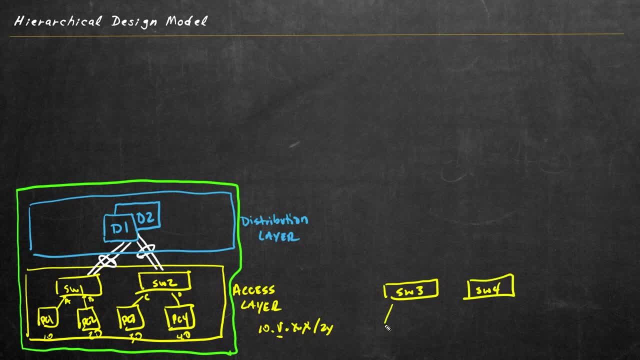 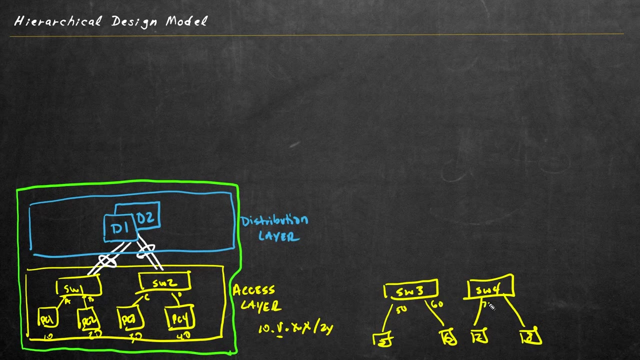 call this switch three and switch four. They've got some devices that are using these switches to access the network. We'll call them PC5,, 6,, 7, and 8.. And let's imagine that we have four different VLANs over here, Let's say VLAN 50,, 60,, 7, and 8. And we're going to call this switch. 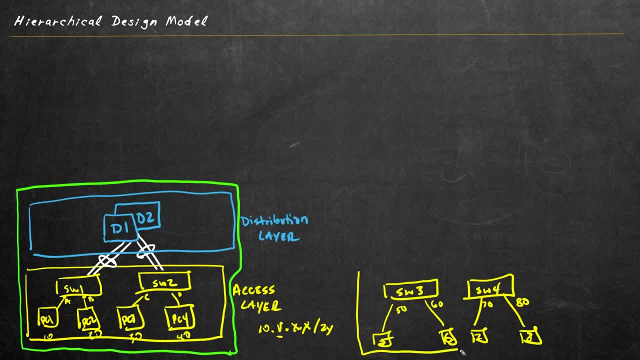 7D and 80. And for the second location, the second building, this would also be referred to as the access layer And, just like in the first building, we also need something that can route between those VLANs. So we have a distribution layer switch D3 and D4, and we've 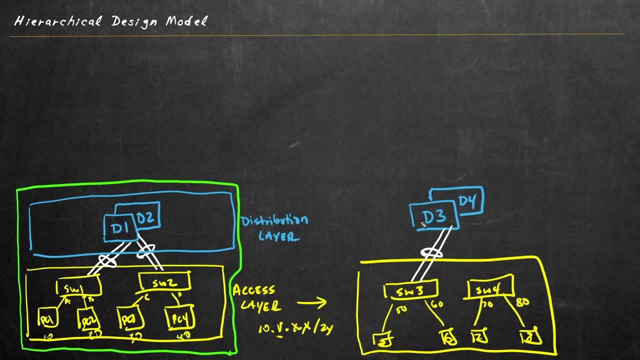 got some fault-tolerant cabling and connectivity between that pair and the switch three and also some fault tolerance and connectivity between switch four and those distribution layer multi-layer switches. So for the second building that would be their distribution layer, And let me 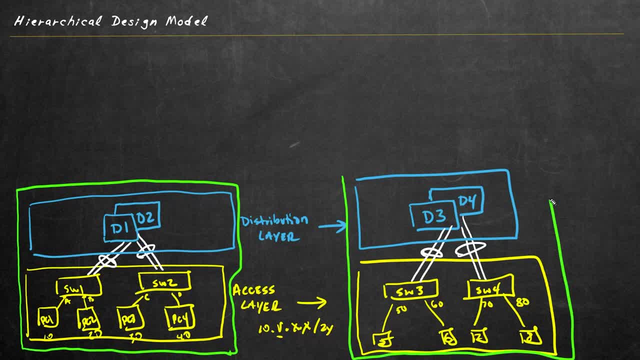 add a whole rectangle around that to represent all the stuff at the second building in this campus design. So it's important to note that between these two locations we have some high speed connectivity. It's available to us either fiber or copper, but it's not going over a slower 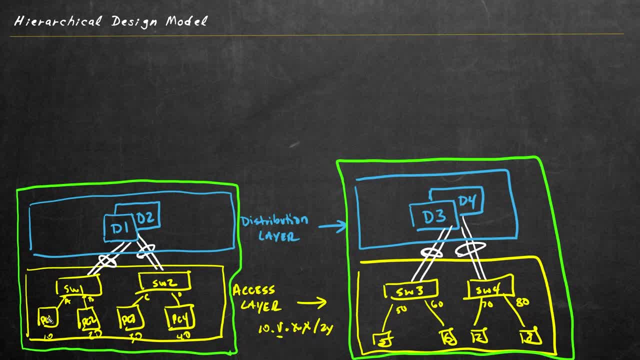 wide area network connection. So the key here is: what if a PC over here on the 1010 subnet in VLAN 10 needs to access a device over here in VLAN 50, which is the 1050 subnet? Well, our challenge is: 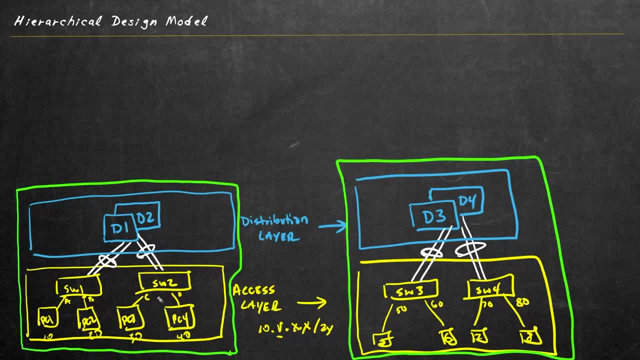 that over here in this section, they can all route and forward, connect to each other. So we've got a lot of traffic between each other And over here they can do the same. We have nothing yet that's allowing the connectivity between these two buildings. So here's what we do: We get some. 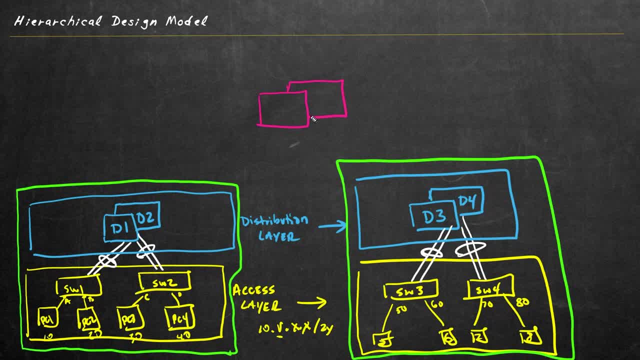 more devices that are going to provide that connectivity And I'm going to draw two for fault tolerance here And this is referred to as the core layer. So I'm going to label these as core one and core two And let's draw some connectivity, We'll make some fault-tolerant. 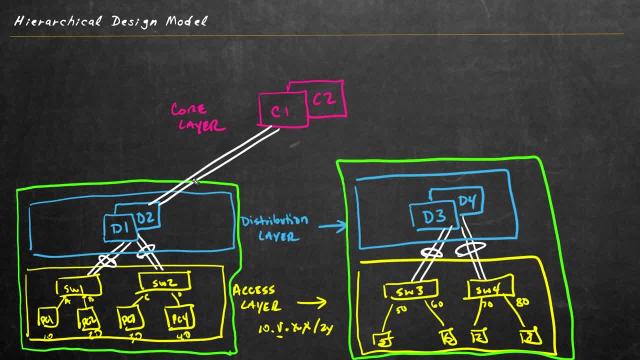 connectivity between these distribution devices here and the core and the same over here. And in the old days, like 15 to 20 years ago, when I first started working, they referred to these as switch blocks, So I'm going to call this switch block number one. 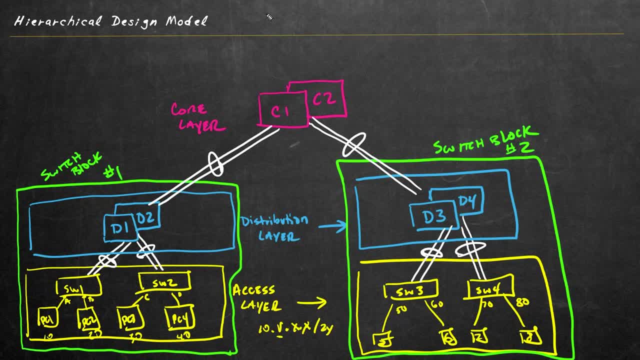 And over here I'll call this switch block number two, And this is commonly referred to as the three-tier hierarchical model, And the intent is for this to be scalable. So if we have a campus, for example, with 20 or 30 buildings, we could just create additional switch blocks. 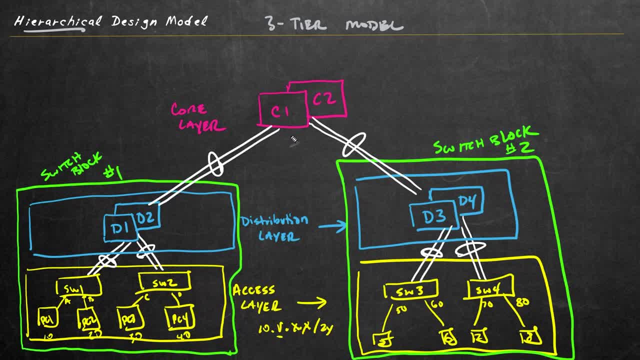 at each of those locations and then tie them together with our core. So let's take a moment and talk about whether the core should be layer two or layer three. If the core is layer two, which would make D1 and D2 effectively in the same subnet as D3 and D4 with each other- 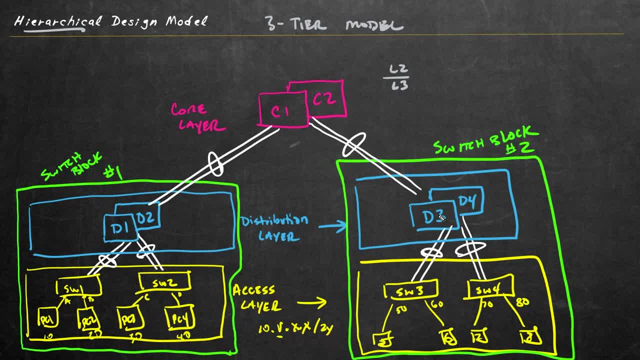 With OSPF. they can become OSPF neighbors, no problem. Learn about the routes and reachability and forward traffic, no worries. However, if we had like a hundred different switch blocks that we're all gluing together with the core, if it was layer two, that means that the distribution 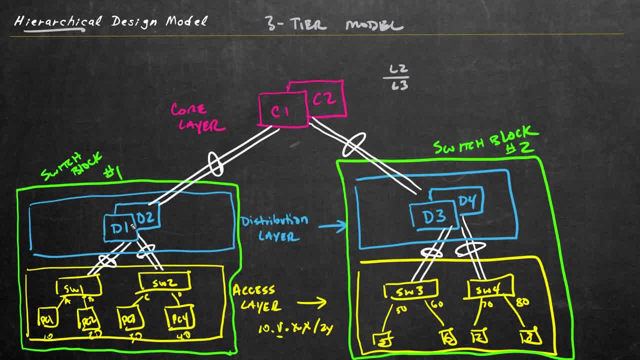 devices here would have maybe 99 other peers or more, depending on how much fault tolerance we have in those other switch blocks, which having 99 peers on all of them, would be a lot more of overhead. So if the number of switch blocks is growing, are you expected to grow? We could. 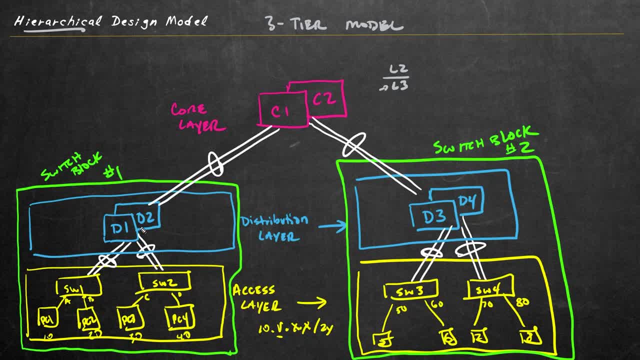 use a layer three core instead And that way the distribution layer devices in each switch block, for example switch block number one, they would peer only with the core at layer three and they wouldn't have to peer with the other 99 switch blocks and those distribution. 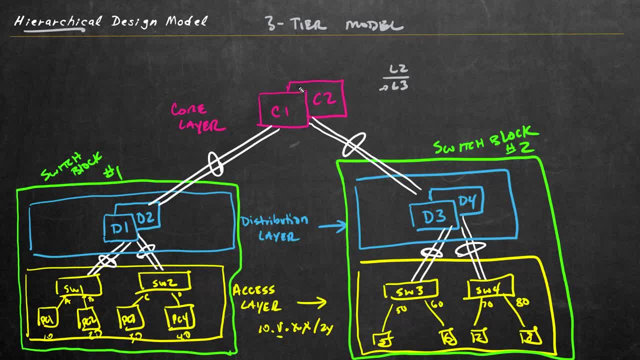 layer devices that are in those other switch blocks. So we'd have some more work here at the core because they would have to peer with everybody. but we wouldn't be putting that burden on every single distribution layer and the routing function there. So as a general rule we're going to do a layer two core if we have a small number of blocks and a 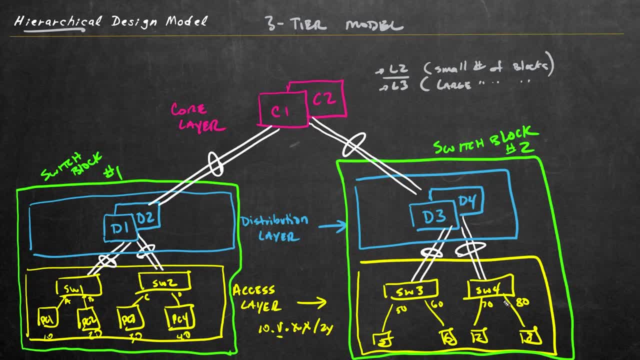 layer three core if we have a large number of blocks, So at the axis layer in these switch blocks. these switches switch one, two, three and four. they are layer two forwarding devices with trunking up to the distribution layer At the distribution layer. these are multi-layer. 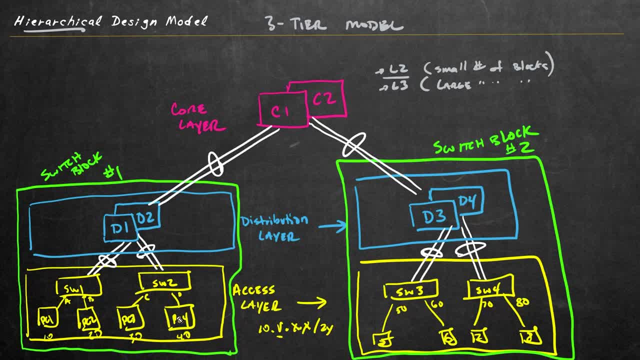 switches with routing capabilities between the various VLANs. They can also peer and route with either the core directly, if it's layer three, or other switch blocks, if it's layer two, at the core, And then the primary purpose for the core is just high speed connectivity. So let's take a look at 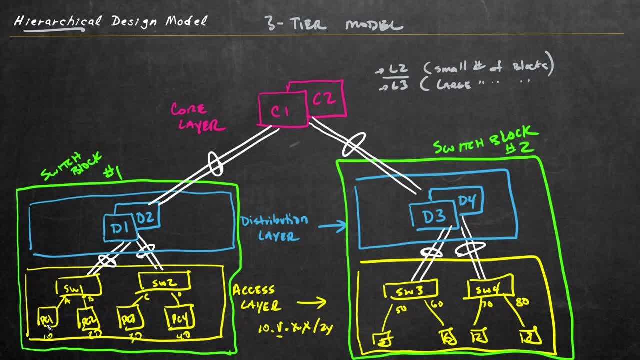 the next logical step. That is well, what if PC one right here in the bottom left hand corner? what if it needs to go out to the internet? or what if it needs a company server? Where do we put those? And the great news is, we can create logical blocks for those as well. So let's imagine: 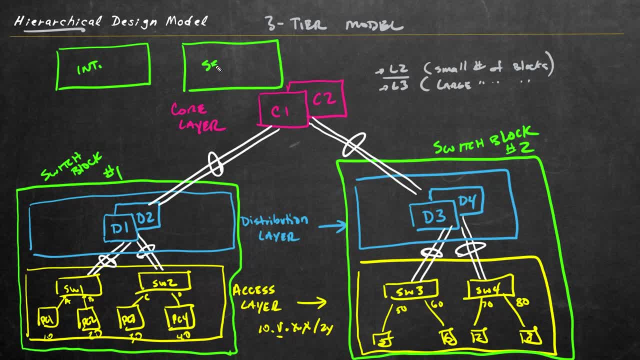 this represents the internet and this represents the company servers. So we'll put some kind of a routing device on each of those, which could be a multi-layer switch or a typical router, and some fault tolerant connectivity to the core, And then any clients need to actually 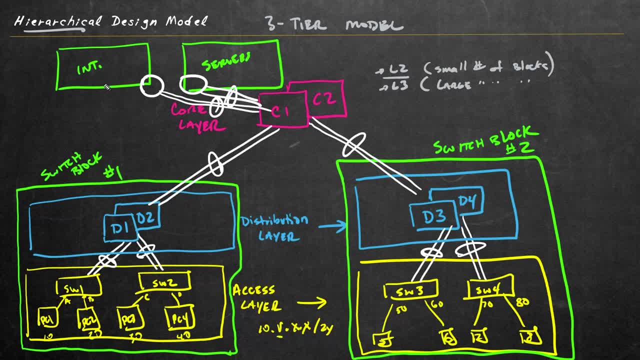 access out to the internet. We've got connectivity from the core out to the internet as well as for company servers, So we might have NTP and DNS and web services and DHCP services et cetera. They're all located here And no matter how many switch blocks we add, we have like the same number. 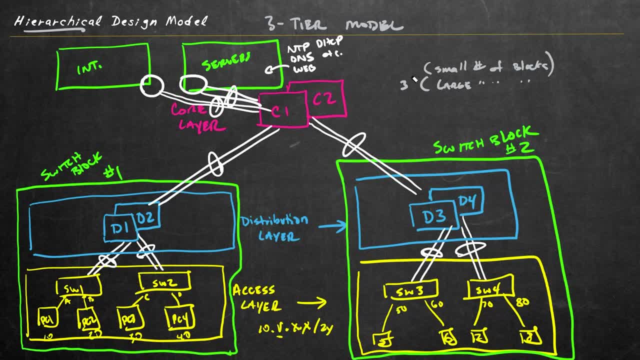 of hops between a switch block and those resources. So let me clean this up just a little bit. And this represents a three-tier hierarchical model with the access layer, distribution layer and the three tiers in the three-tier model. However, what if you're a smaller company? And I'll go ahead. 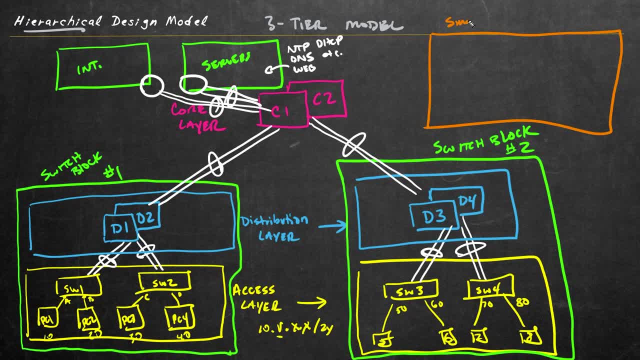 and do a little block around here for a smaller organization- And when I mean smaller, I'm talking about something that's not a huge campus environment- We still have our devices that need to access the network, So these are PCs. We call it PC one, two, three and four. They are still. connected to layer two switches And that still is referred to as the access layer. That doesn't change And we still need some routing functionality that's going to be able to route between those. So we'll call this D1 and D2 in this smaller environment And we'll put some connectivity. 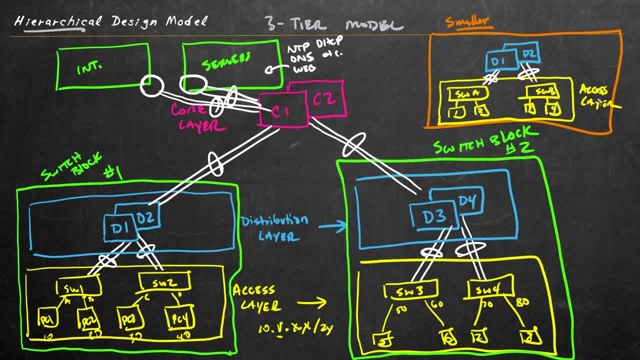 there with some fault tolerance, Very good. So let's imagine that we had no other blocks to connect to at the smaller company. We really don't need to have a core or a separate core to route between this grouping of equipment and resources and something else at the company, because there. 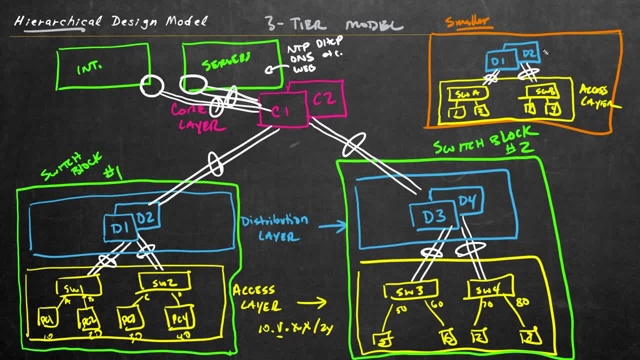 is nothing else at the company. So what we could do is we could double up with this functionality and we could put right here C1 and C2.. It's the same device, the multi-layer switch, that's going to be providing the functionality of the other devices, And that's what we're going to do. We're 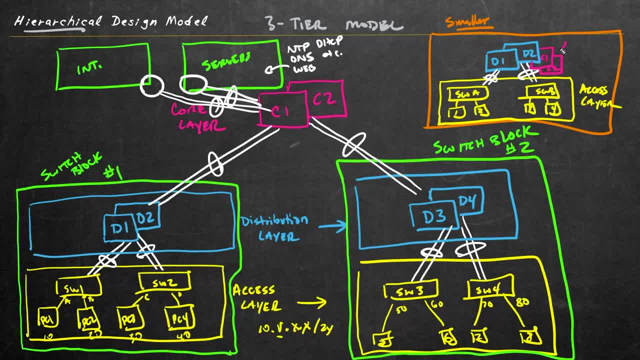 going to go ahead and draw a rectangle around that And I'm going to use both colors And so, if we count the layers here, we have one layer there, the access layer, And then we have a second layer here for this, And we're going to go ahead and draw a rectangle around that And I'm going to 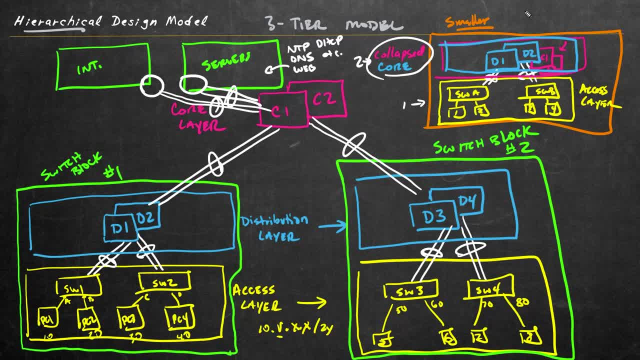 go ahead and draw a rectangle around that, And that's what we're going to do. We're going to go ahead and draw a rectangle around that And this is a distribution core- that are combined together And this is an example of a two-tier hierarchical model. So the three-tier is fully. 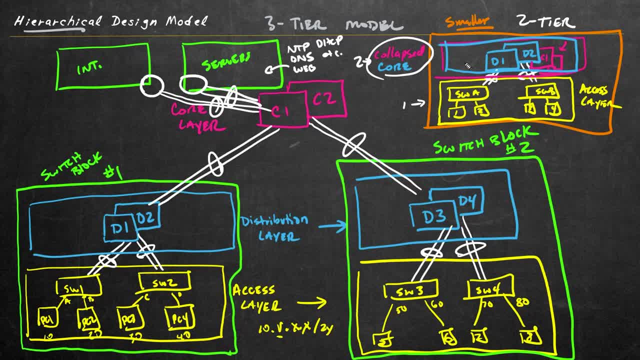 separate devices for access layer, distribution layer and core, where a collapsed two-tier model simply has the distribution and the core collapsed or integrated together. So here at the collapsed core, we may still have separate logical exit points for things like the internet or company. 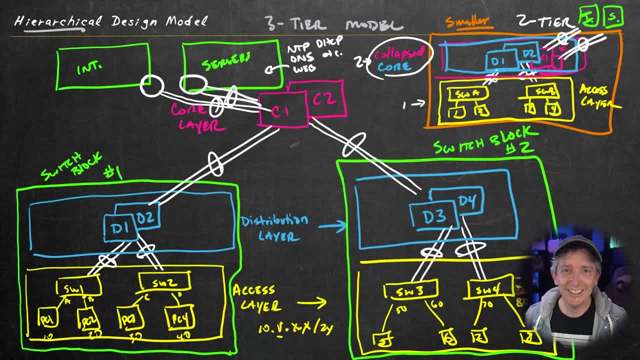 servers And that connectivity would be directly from this collapsed core. So as I was putting my thoughts together about chatting with you about this two-tier and three-tier, I was able to three-tier hierarchical model. I thought you know what. Let me put this together in action. 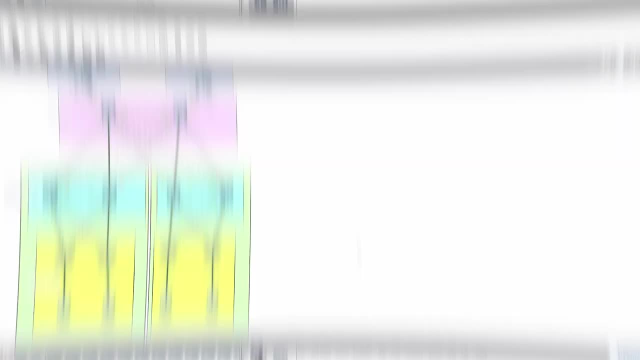 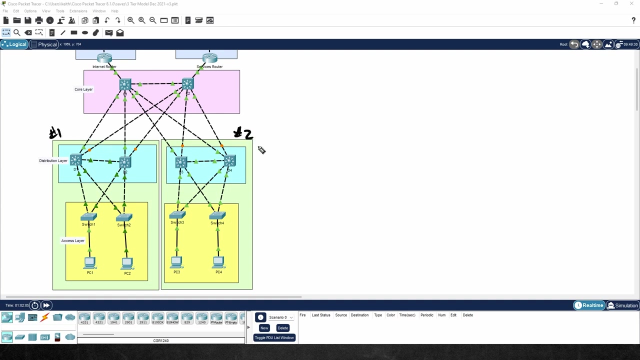 in Packet Tracer. You want to see it? Let me show you. All right, And here we go. I've got two switch blocks. I've got block number one here on the left and number two here on the right, And in switch block one I have a couple of access layer switches and a couple of devices. They're 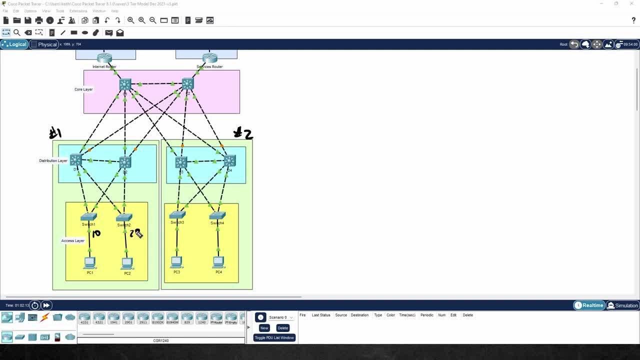 in both different VLANs. This guy is in VLAN 10.. This guy's in VLAN 20.. And over here in switch block number two, this is VLAN number 50 and VLAN number 60. And that's the access layer for both. 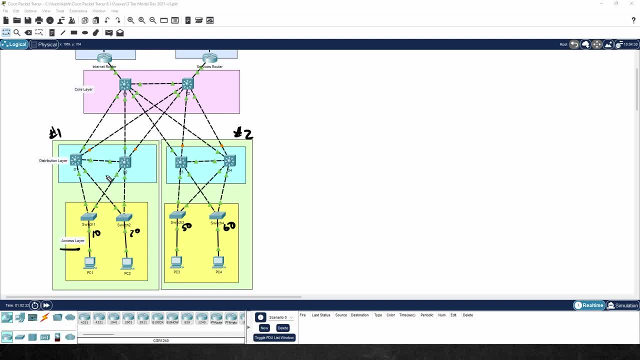 of these. And then we've got the aggregation here at the distribution layer which is performing routing. These routers are performing routing locally here in the switch block between VLAN 10 and VLAN 20.. And in switch block two these routers here at the distribution layer are: 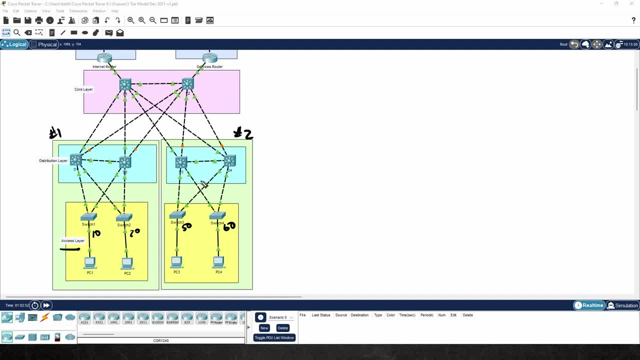 providing routing between VLANs 50 and 60. And if we need connectivity between these subnets here in switch block one and the subnets here in switch block two, that's where we use the core layer. So the core is what's providing connectivity between these two switch blocks. So in my 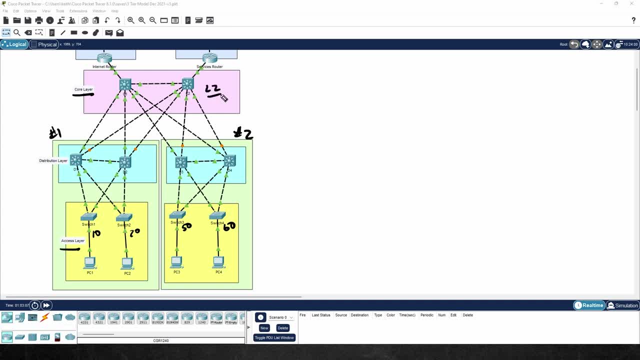 implementation here because it's fairly small. I'm just using a layer two core And I'm using VLAN 777 for the connectivity between the distribution layer devices in each of the switch blocks. So VLAN 777 is used explicitly for the core connectivity and 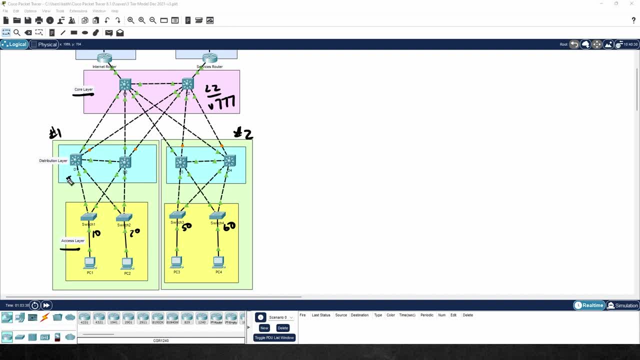 VLAN 777 is not allowed down here. So on these trunks going from the distribution layer devices down to the access layer devices, I've excluded, on these trunks down here I've excluded that specific VLAN. So these switches down here don't have any clue or knowledge about VLAN 777.. That's. 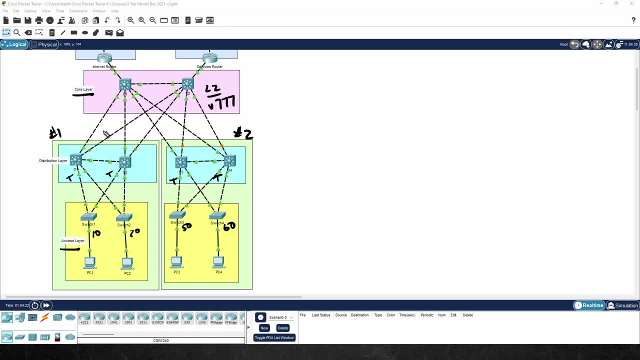 why I'm using these distribution layer devices and these distribution layer devices. So then I have routing protocol set up between these distribution layer devices over the layer two core, So the distribution layer devices can dynamically learn via routing protocol how to forward to non-local networks. That way D4 can learn about how to get to the 1010 subnet. the 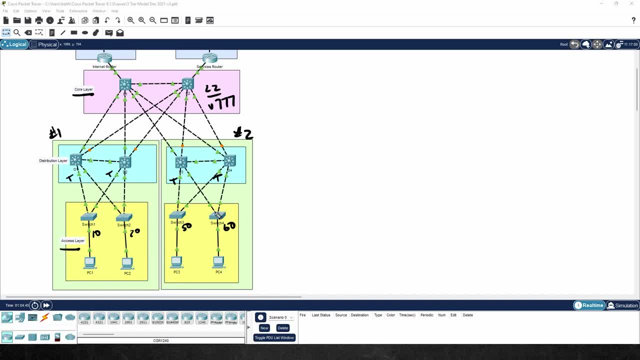 1020 subnet and vice versa. D1 and D2 can also dynamically learn through a routing protocol on how to forward in the direction of the 1050 and 1060 subnets which, in this diagram, are being supported by VLAN 50 and VLAN 60.. 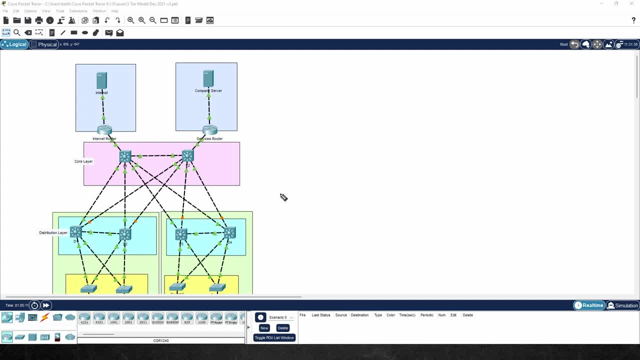 So let me scroll down a little bit and let's talk about a little more of this topology. So if a user in any of those VLANs needs to go out to the internet, we also have reachability out to this block that represents the internet. So if we had dozens of switch blocks, so this is one, this is. 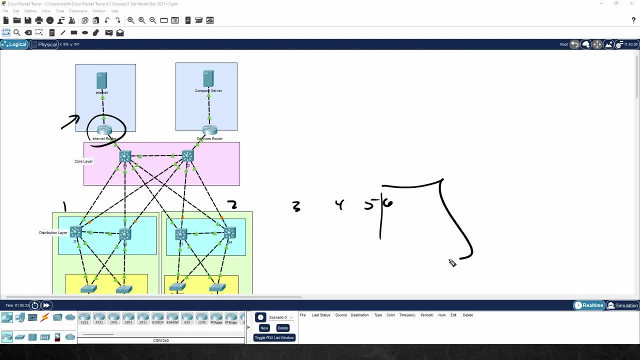 two, and let's say we have three and four and five and six, the person that's in the sixth switch block and end user down here at the access layer. if they want to go out to the internet the traffic would go from the distribution layer in their switch block through the core and up to this. 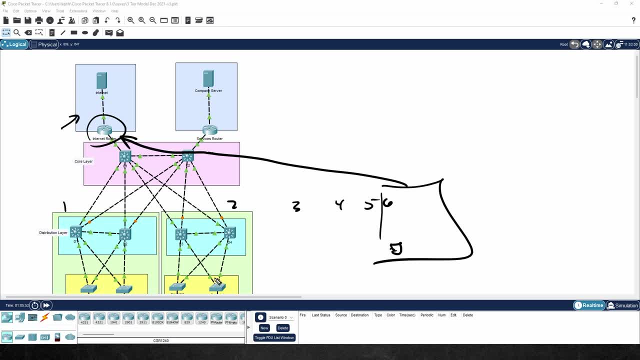 section which represents the internet, which is much better than having to go through the 10 different routers to get there. This way, every switch block has equal access regarding the number of hops, for example, to get from that switch block in the distribution layer out to the 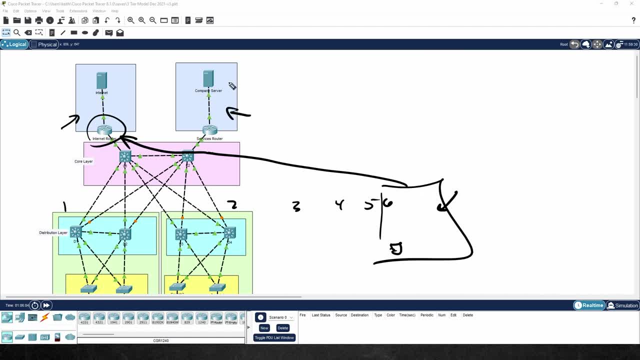 internet, And the same is true for access to company servers. So we might have a server here at 10.90.0.100, and perhaps the server is providing DHCP services and web services and NTP et cetera. We could configure all those services here and then on the logical layer, three interfaces they're. 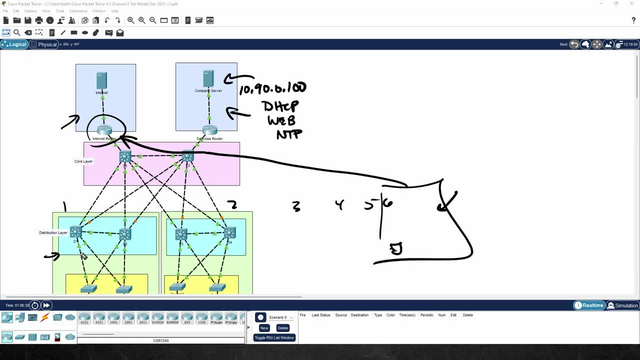 supporting the access layer. We can put IP helper enable DHCP forwarding so that clients, when they make a DHCP request, that request can be forwarded up to the DHCP server who can pick from the appropriate pool based on where that request is coming from And then, when it responds back as a 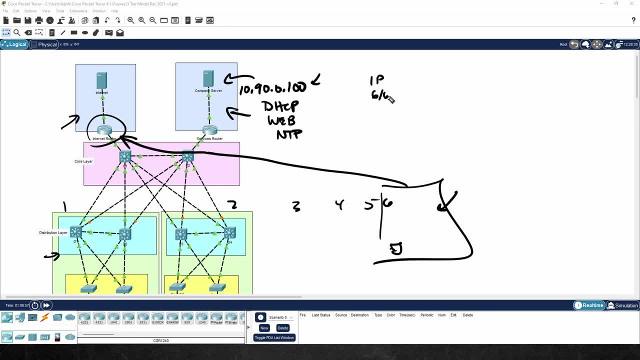 DHCP server. it's going to hand out IP addresses, default gateways, which, by the way, for fault tolerance, we'd want to make sure that if any of our distribution layer switches fails, the other one can take over. So very likely, here we're going to be running some kind of a first hop redundancy. 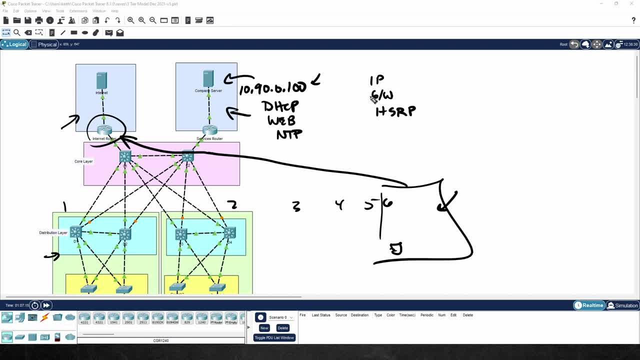 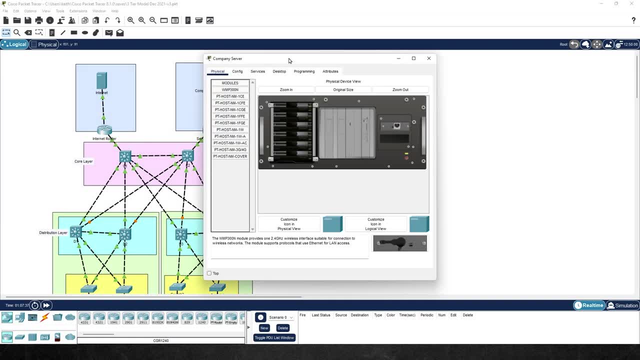 protocol Like HSRP from Cisco, And that way when we hand out the default gateway, we can hand out that virtual IP address associated with the HSRP group. So as a quick test, let's go up to this company server for a moment and click on services and go to DHCP. Yeah, sure enough, it's got scopes, or? 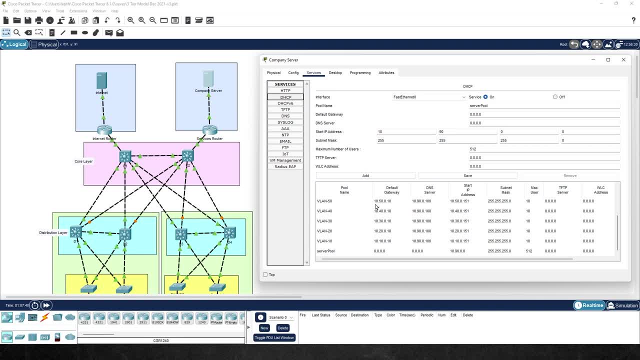 pools of addresses for the 10.10,, 10.20,, 10.30,, 10.40,, 10.50, et cetera. So it can hand out IP addresses And if it hands out an IP address for VLAN 10 and the 10.10.0 subnet range, the default. 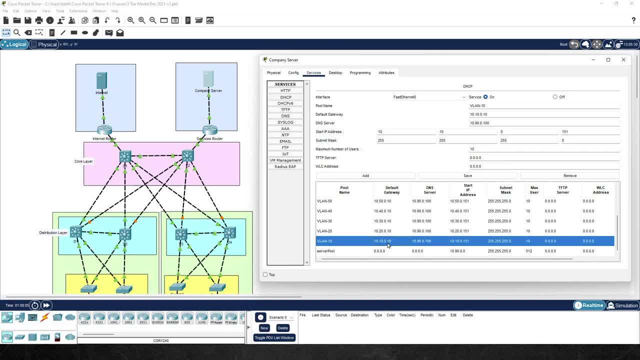 gateways it's going to hand out is .10.. And that would represent the IP address for VLAN 10 and the 10.20.. And that would represent our HSRP virtual address that we're supporting on these distribution layer switches, And up here I have one server representing the internet. Let's take 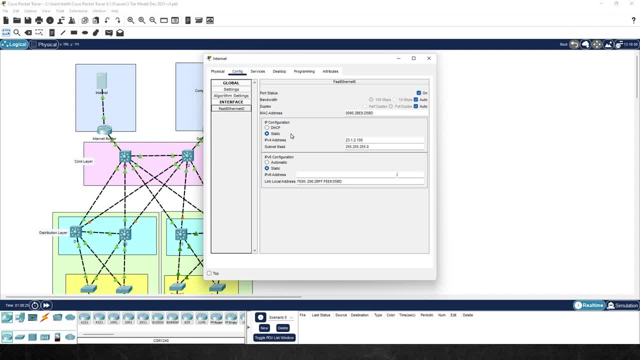 a look at what his address is. So we've got a config and fast ethernet. So I set up this one server at 23.1.2.100, just to represent the internet, Although in this lab topology it's just one server representing the internet. So if we tested this, let's go down to PC1 and just hover. 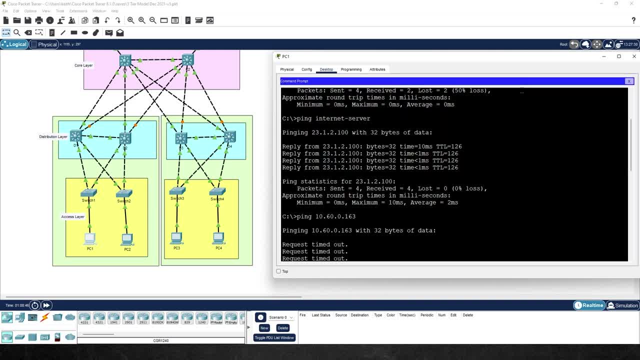 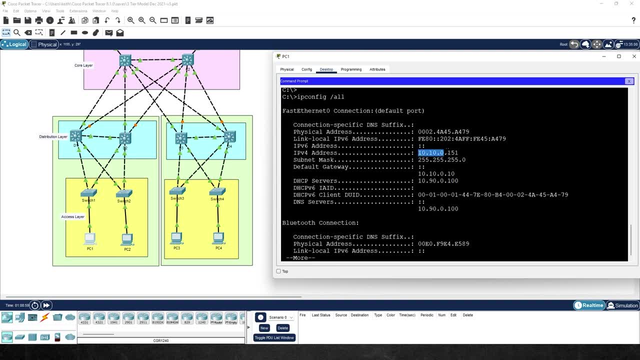 there for a second. This says that PC1 has an address. So at PC1, let's go to a command prompt. So here at PC1, let's do an IA. So this says it has an IP address of 151 with a 24-bit mask. The default gateway is 10.10.0.10,. 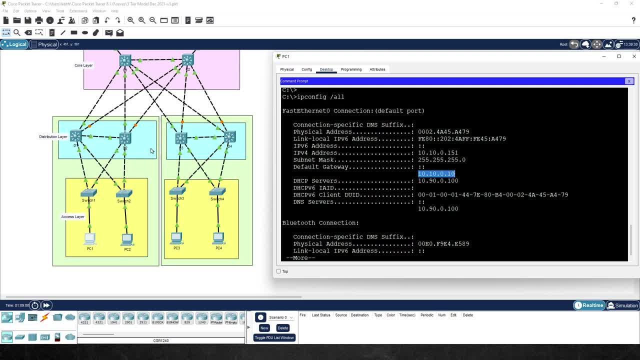 which is an HSRP address being supported by both D1 and D2.. And the DHCP server that gave this client's IP address is 10.90.0.100.. That's the top right server we looked at a moment ago. 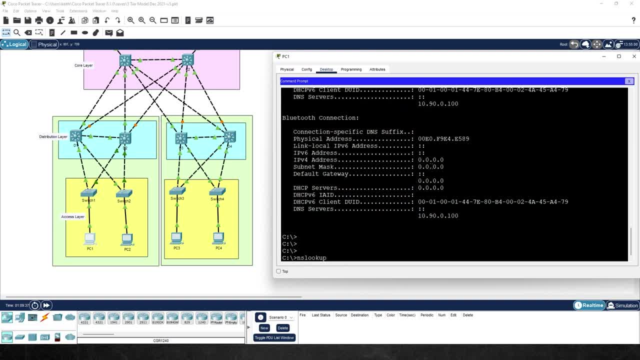 And he also handed out himself as a DNS server. So if we did an NS lookup- I didn't realize that was simulated here in Packet Tracer, but it is- So- NS lookup, let's go ahead and do a internet server, press enter and it comes back with that. 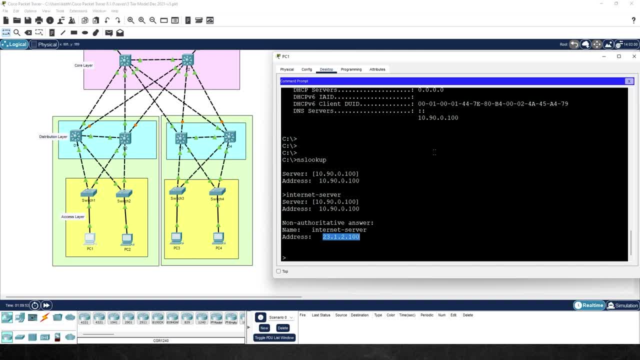 address. So those are DNS requests that we're making up to our DNS server. So I'll type in exit and let's do a ping to internet server, which is our server on the upper left, And yeah, we got connectivity- Fantastic. Which also implies: 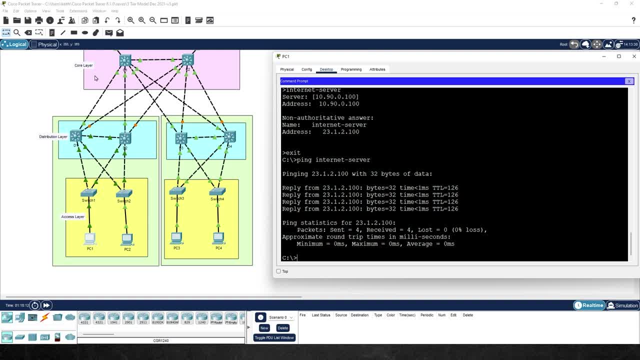 that we have some network address translation that's in use up at that internet block. So before traffic goes out, we're doing source address translation And if we go to one of our distributional devices, let's go to D1 here for a moment. 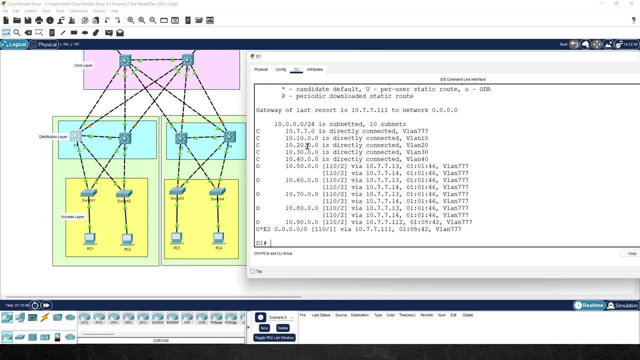 And we do a show IP route. Here are its OSPF learned routes, including a default route which says: if you're not sure what to do, go ahead and forward it to 10.7.7.1.1.1.. That next top represents this guy right here. 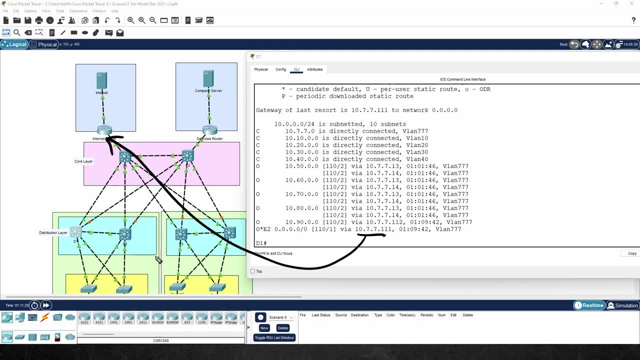 That leads off to the internet. So in putting this together in Packet Tracer, let me just do a quick summary of what it gave me: the opportunity to practice and rehearse and get better at, Even though at double CCIE, the more times you lab stuff up and configure it, 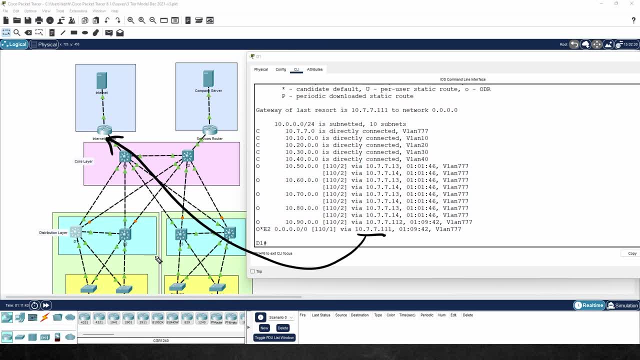 the better you're going to be at it. You're going to get better at it. You're going to get better at it. You're going to increase those skills. So if I can do it, you can do it. So here are a few of the topics from the CCNA blueprint that I had the opportunity to practice. 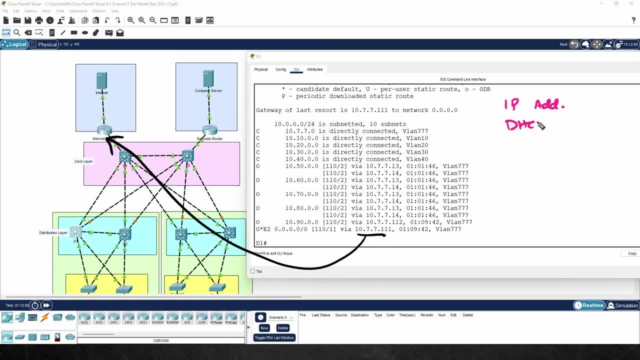 as I put this together: One was IP addressing, There was DHCP, There was DHCP relay, There was layer two stuff including trunking and access ports. There was some first hop redundancy protocol. There was DNS and that FHRP was HSRP- That's the flavor I used. There was OSPF. 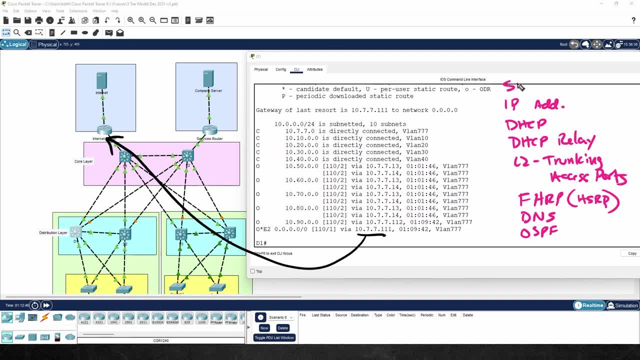 which I'm using for my dynamic routing protocol. I also tweaked spanning tree Because I wanted to make sure that the appropriate devices were the root of the spanning tree, with C1 being the root and then C2 having a artificially lowered priority So that if C1 goes away, 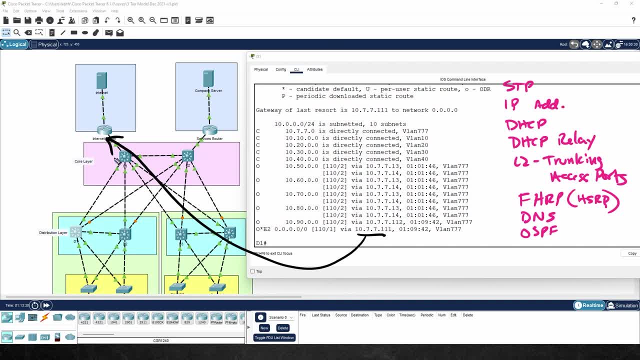 C2 would become the root of VLAN 777, which I'm using for my core connectivity between the distribution blocks. I also had the opportunity of playing with NAT network address translation, specifically port address translation, And that was right here at this router as traffic. 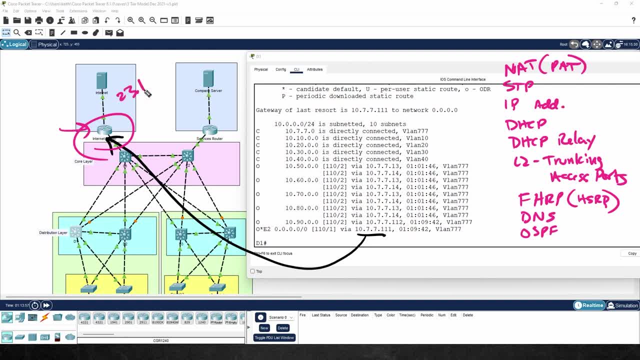 is being forwarded to my little pseudo internet right here, which is the 23.1.2 network. So it looked and felt like I had the opportunity to play with- I don't know, maybe 10, 15% of the entire blueprint and building this three tier hierarchical design with the core. 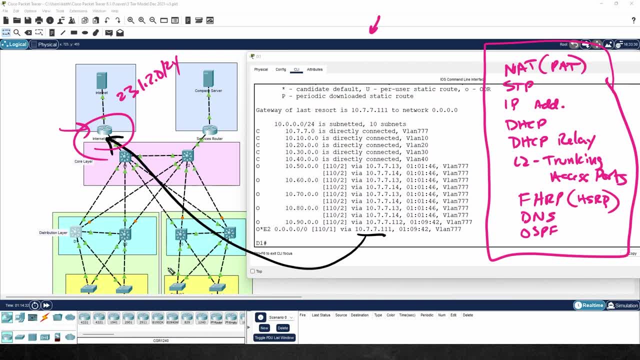 the distribution layer and the access layer. So I'm going to go ahead and save this topology here in packet tracer and I will put it up on my site So anybody who wants it can download it and play and practice with it. And the website you can go get this at is the Keith Barkercom. 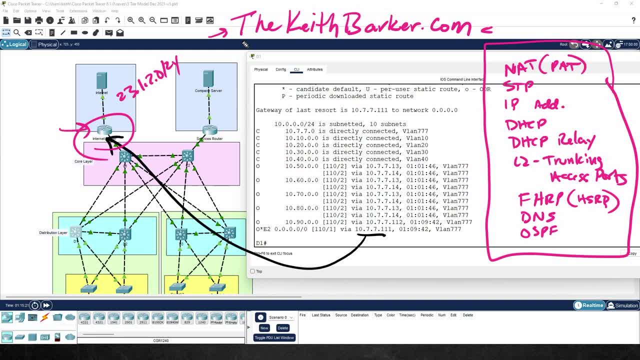 And it'll be the one labeled three tier hierarchical model. So if you'd like to download it and take a look at this and play with it, you're welcome to. I would also encourage you, once you've taken a moment to think about the three layer hierarchical model, to go ahead and 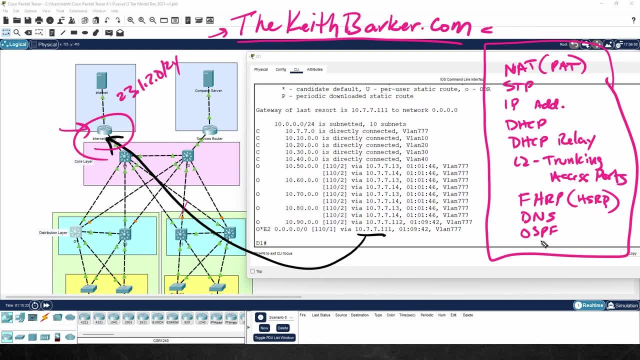 build your own, And that'll give you the practice with all of these technologies, Should you want to get better at them. In fact, my challenge would be download this, use it as a reference and then set it up on your own from scratch, And then, if you get stuck or have a question, 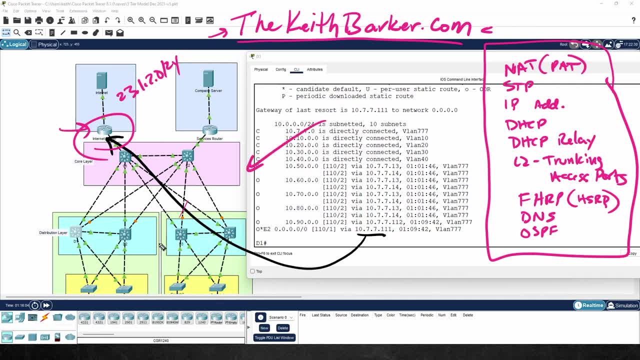 you can go back and look at this design here, see what I did and then keep on pressing forward. Also, join me if you're studying for CCNA or you want to just refresh your skills about machine learning, And I'll see you next time. Bye. 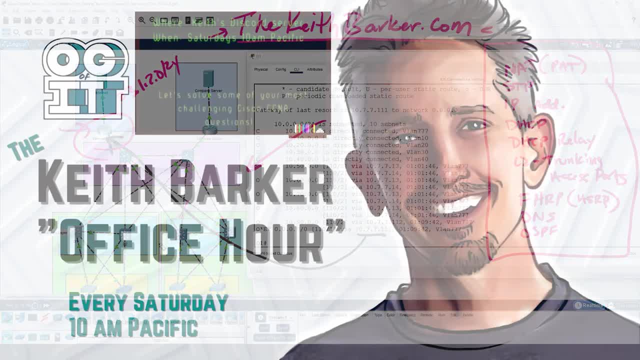 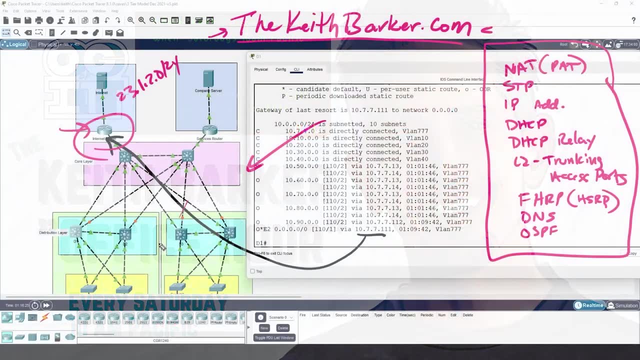 the concepts associated with CCNA. Join me every Saturday at 10 o'clock AM Pacific time on my discord server for my free and open office hour, And then every Sunday we have a follow-up quiz online on YouTube, and that's at 11 AM every Sunday Pacific time. We'd love to have you join. 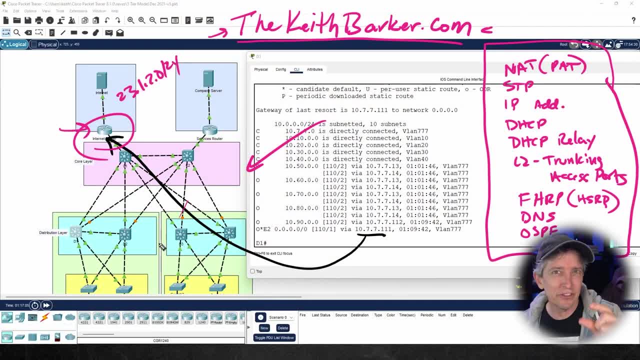 us for each and every one of those events. So thank you for investing a little bit of time to become better at understanding and working with the three tier hierarchical model from Cisco systems, And I look forward to seeing you, my friend, in the next video or live event soon.